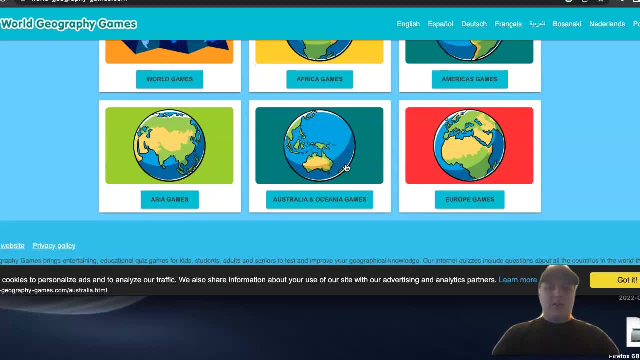 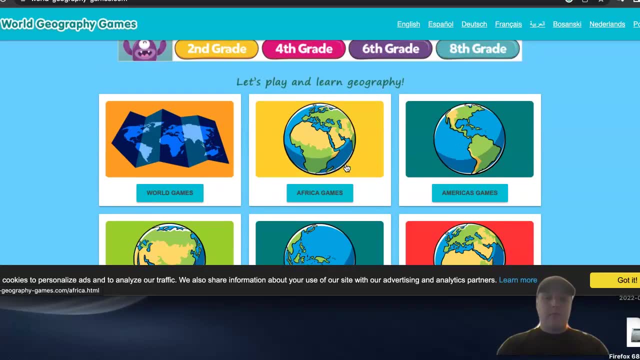 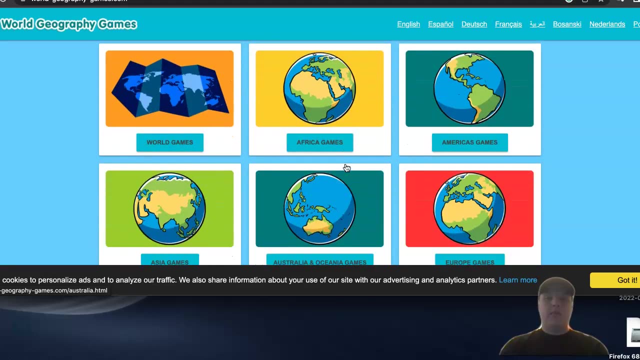 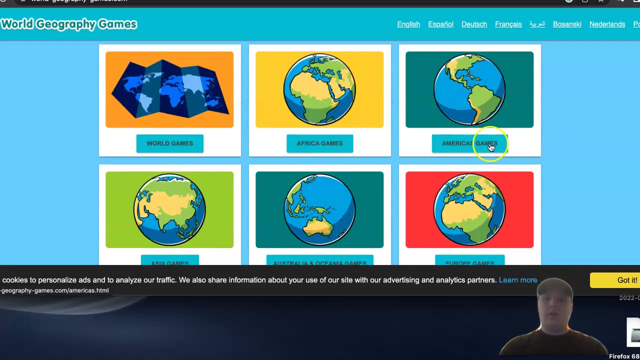 on that And I thought that this website would be a fun way to learn more about what we're going to be learning in the classroom through social studies and world history, And it is perfect because it's already kind of divided- similarly like our units will be So as we cover Africa or America, Asia, Australia, Oceania. 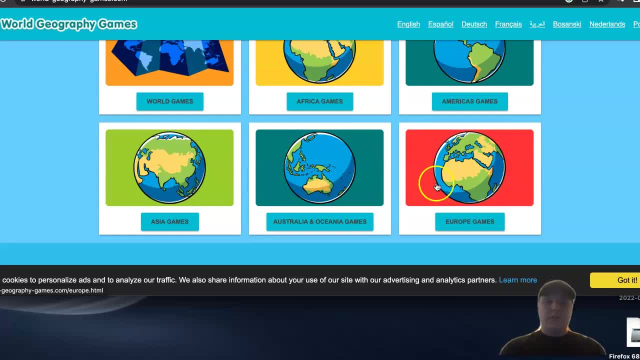 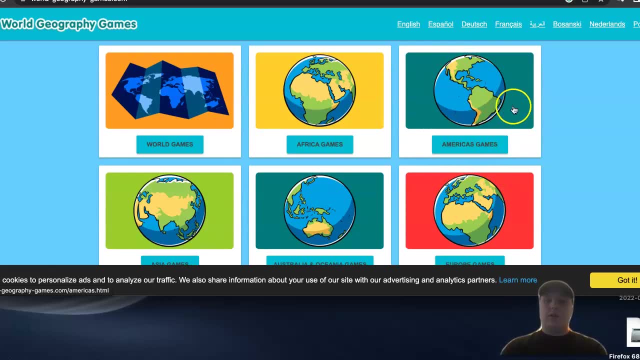 or Europe Through individual units. we can utilize this website to kind of quiz ourselves throughout and at the end of the unit, to kind of track our knowledge and progress, And then towards the end of the semester we could even utilize the world games and kind of tie all of our knowledge together. So we go ahead and and, oh and. 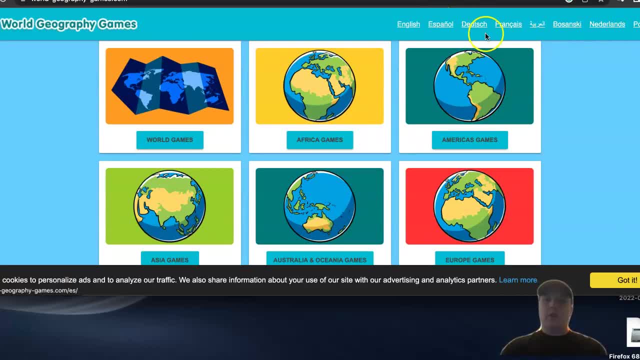 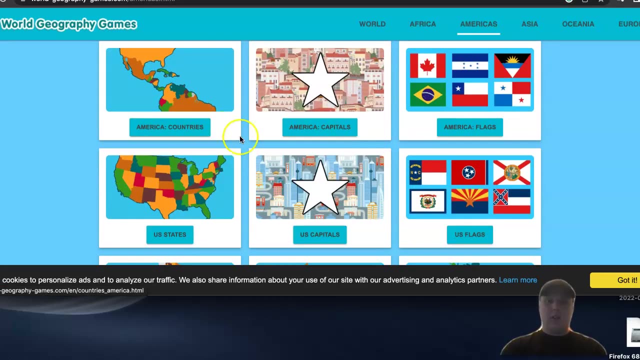 also there. it provides different languages. up here as well. Some of you, you know, could be fluent in different languages, so just a nice tool there. So if we go ahead and click on America, America games, you can see that there's actually quite a lot of games that they 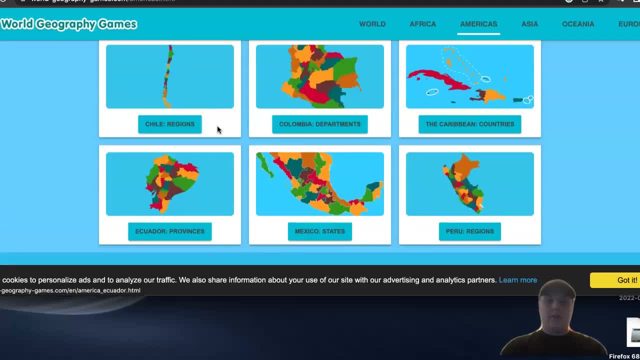 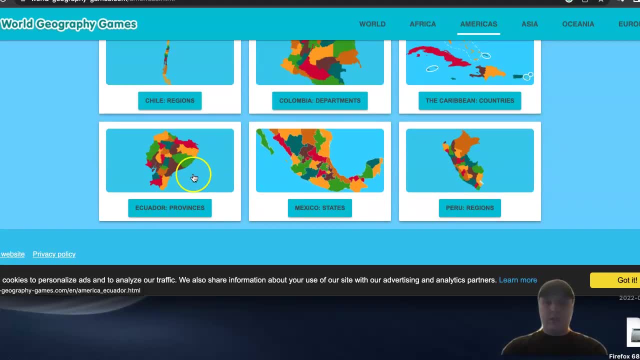 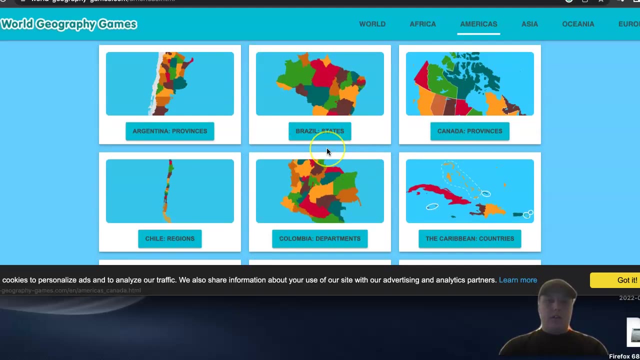 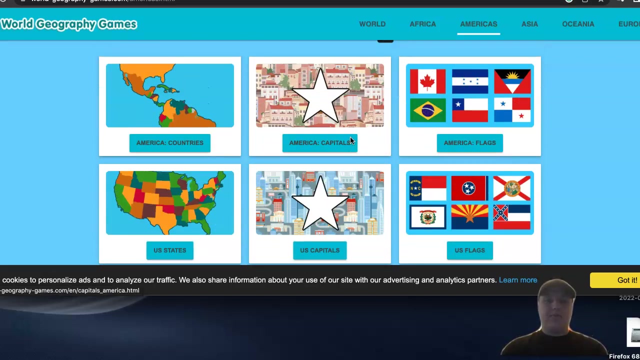 provide that can make it fun for you. So obviously, within this there's, you know, Central America, as you see here, with Ecuador, Mexico, the Caribbean, Canada, So it's not just America, it's, you know, North, Central and South America here. So let's go ahead and 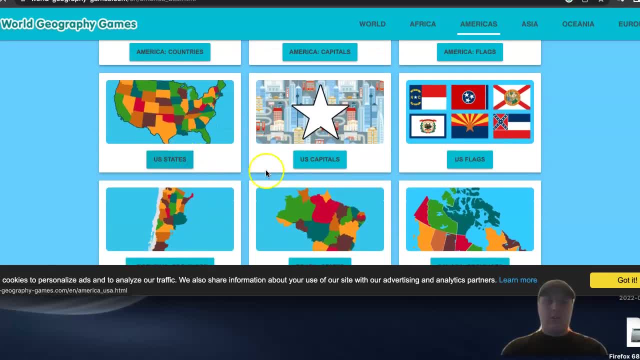 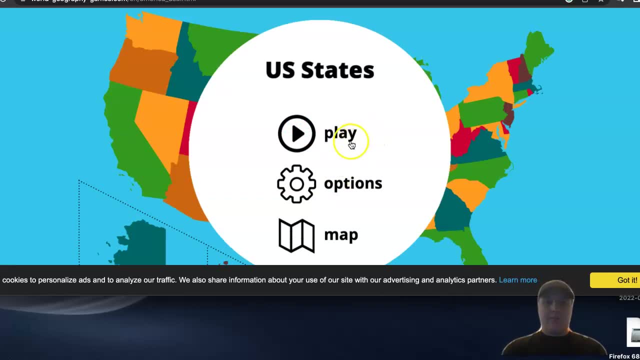 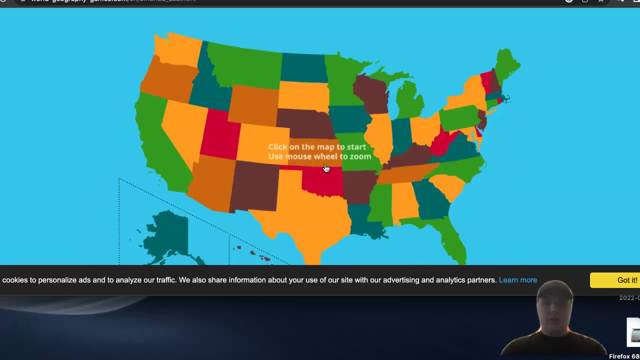 click on one of these. We can just go ahead and click on the US states, Let that load up. We can click, play, Click on the map to start, Then use the mouse wheel to zoom, Just like that. So we'll go ahead and click and start. So Wyoming You know. 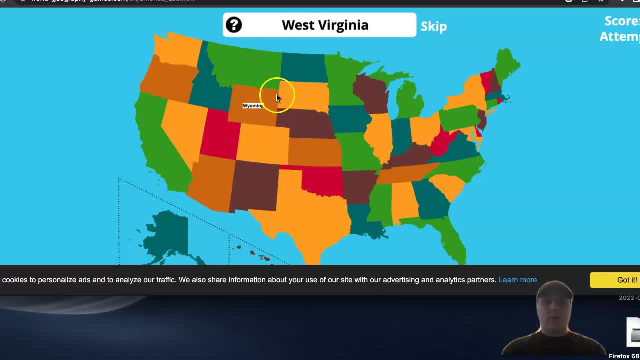 that's right up here, Got that correct, West Virginia. See, that's what happened. when you get it wrong, It'll let you know. All right, so we'll go ahead and correct that, and then it allows you to move on. Then Alaska, Indiana, Colorado, our hometown- And then it kind of shows you: 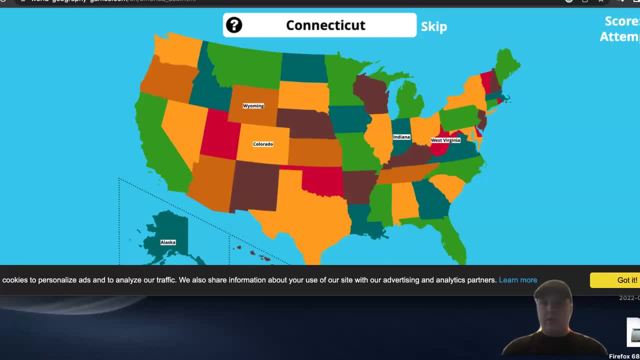 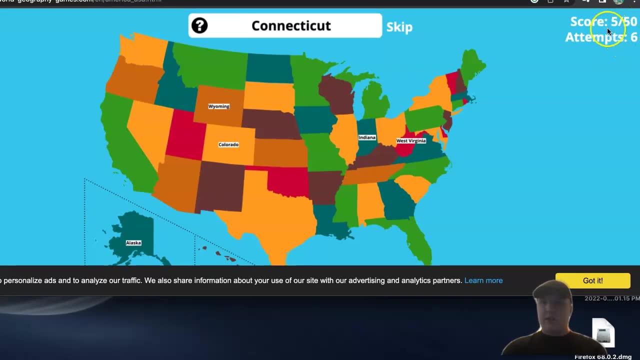 on the right here. I think this green quite shows that. Let's see, I can move that over a little bit. So we have six attempts and our score is five out of 50.. So we have six attempts and our score is five out of 50.. So we have six attempts and our score is five out of 50. 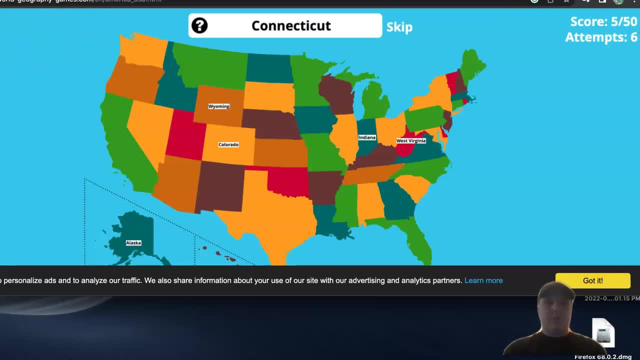 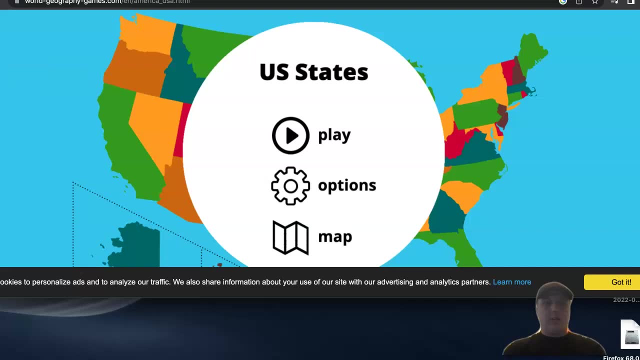 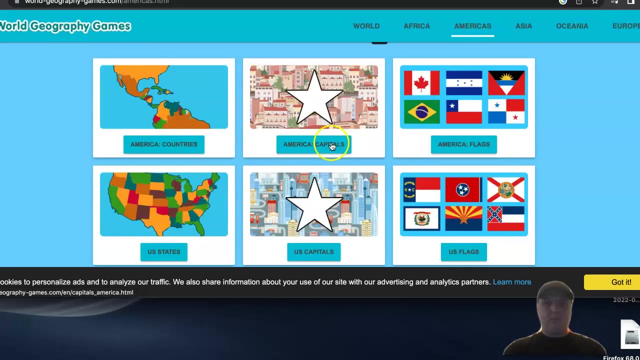 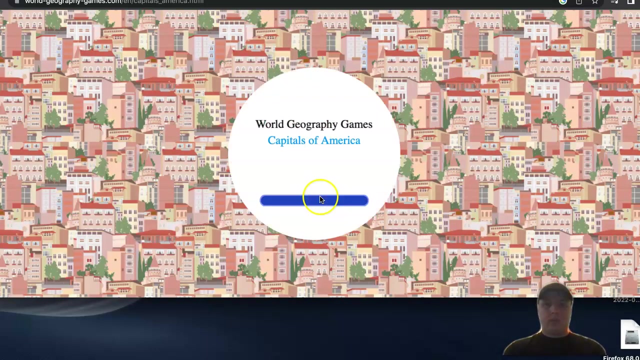 I'll just kind of quiz you until you go through all of the states and finish that up. So we'll go ahead and back out of this so we can show you another one. So if we go capitals here, Let that load up. Go ahead and click on that. 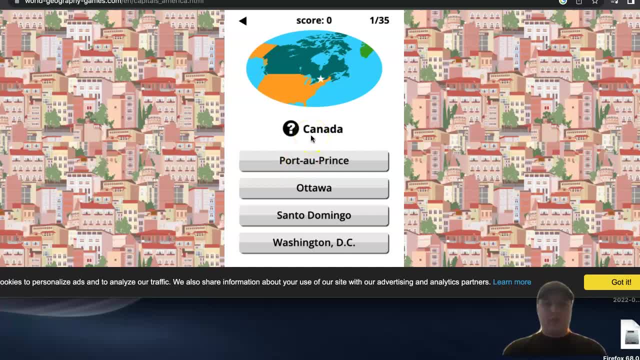 then click play. So it is asking for the capital of Canada. All right, So we have four different options to answer from And you know, sometimes you might not be familiar with all of these, because you know it's gonna include Canada. so North Central, and вы говорите оyer. 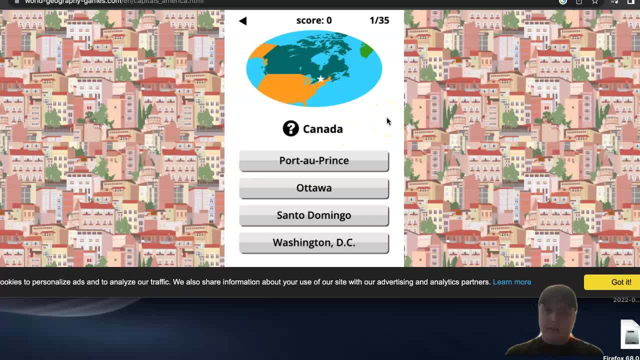 all of these because you know it's gonna include Canada, So North Central and South America, so some of these games could be a little more difficult. but it's always good to challenge yourself and you can always use process of elimination here. so you know Washington DC is in the United States, all right? 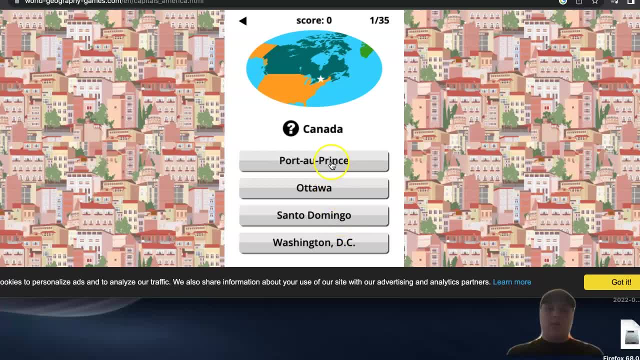 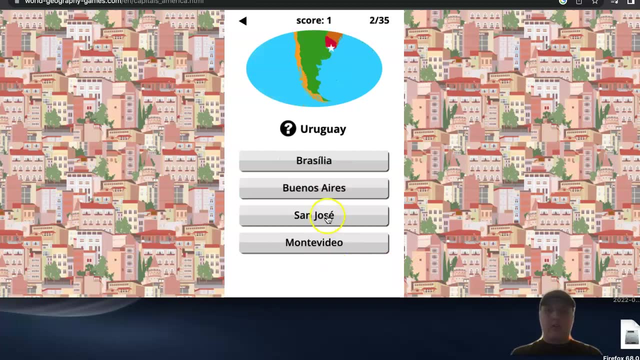 Santo Domingo, Ottawa, Port-au-Prince. so I know that it's Ottawa, so I'm gonna go ahead and click on that. get that little notification out of the way there, okay, so go ahead and click. next, Uruguay, right Montevideo video, Giana. so, as you can see,